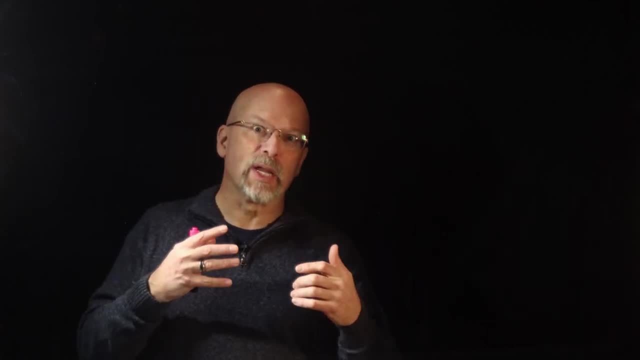 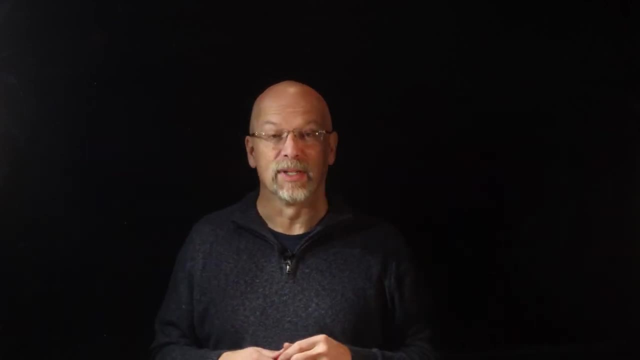 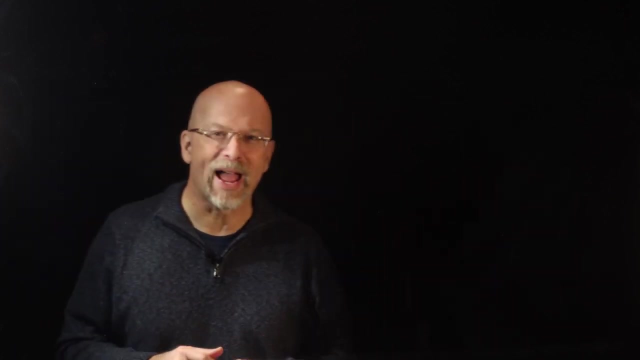 kind of get an idea of, for example, the difference between a home and a grocery store and say, a college, you know, an education building, an academic building, Each one designed by an architect to create a space around people. right, and has create a space for people to live in, to participate in, 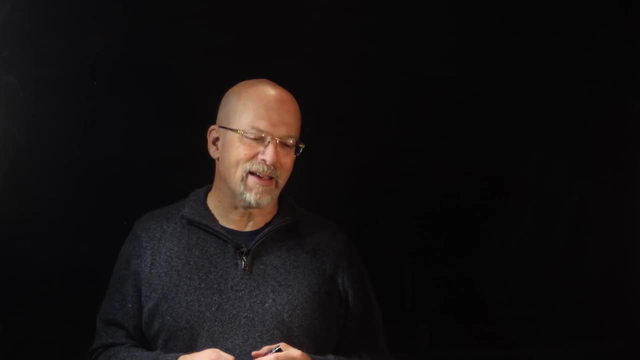 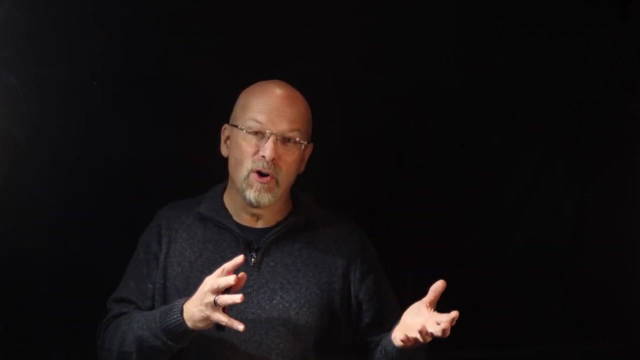 and each one of those spaces well, they have very special purposes. For example, you probably don't have urinals in your bathrooms in your home, right, because that's not the kind of use that you would expect in a in a home bathroom. But whenever you look at the bathrooms in an academic building, 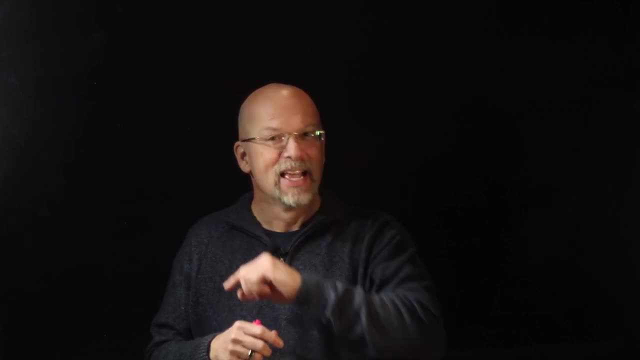 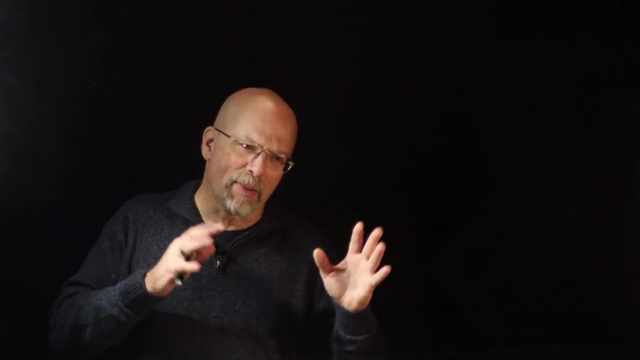 where they expect to have a bathroom. you know you're going to see that the bathrooms and the large numbers of students between classes needing to have a break. well, you're going to have a very different design, but yet the bricks, the cinder blocks, the paint and so forth that is used to 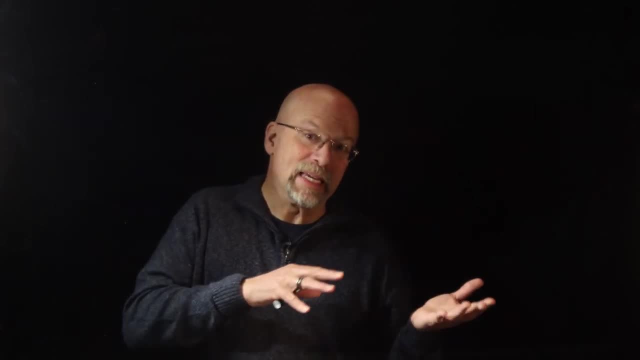 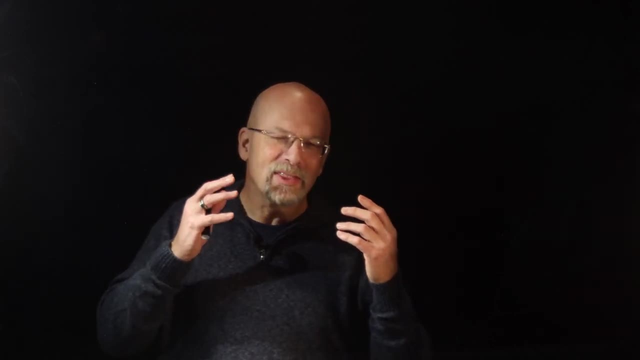 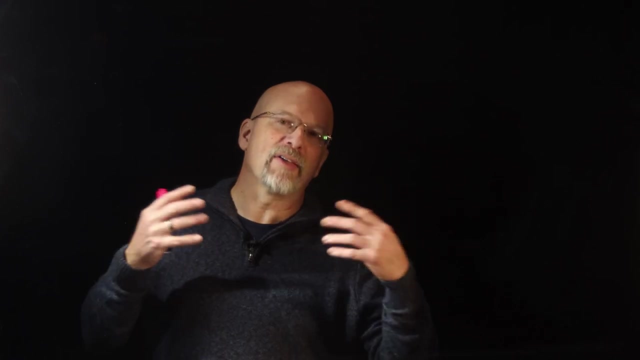 create a home is very similar to the pieces. well, you may have steel girders instead of- uh, you know, instead of wooden studs. but you know, the idea is is that the architect has an idea of the use of the building, how they want things to flow, how they want people to live and use that building. 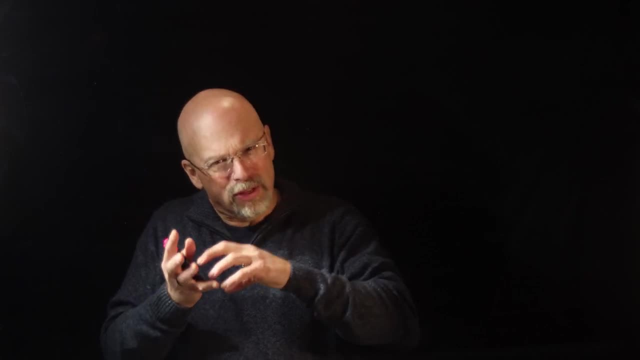 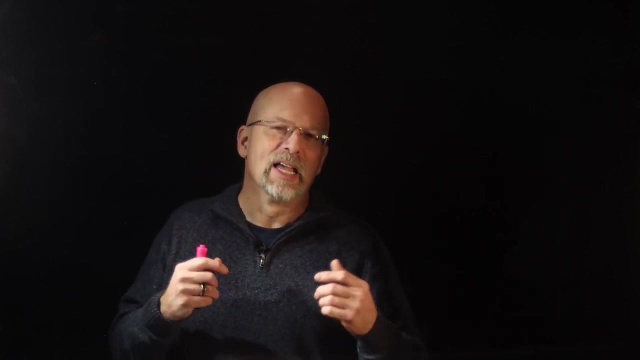 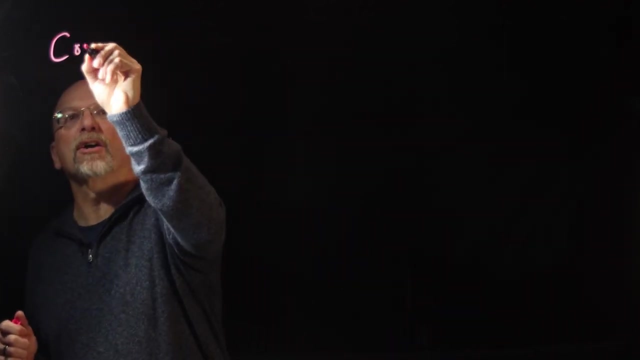 but the components, the, the actual things, the materials that we build the, the building with. that is equivalent to the gates and the circuitry that we've been doing with this computer organization up to this part, so net point. so now what we're going to do is address something called 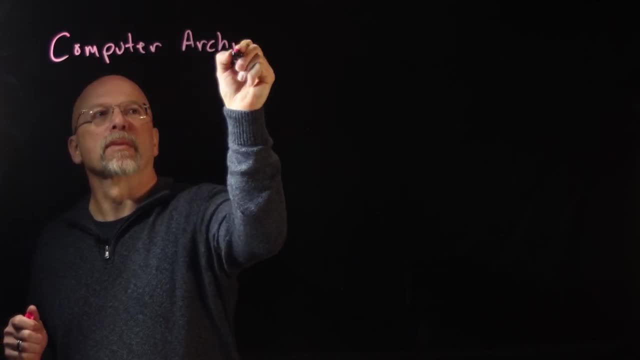 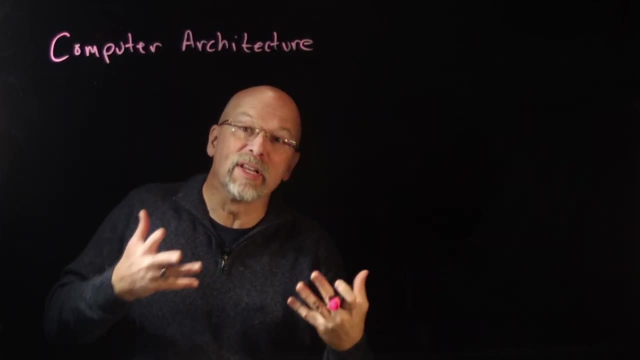 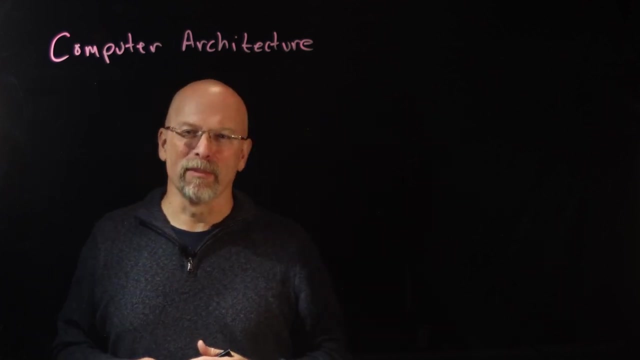 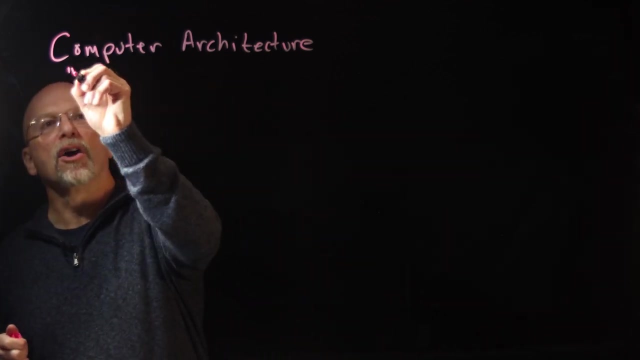 computer architecture, architecture, um, and this is what we have. well, we've been building up to this point where we can build a building. now we need to design the building now. one of the most important parts about computer architecture is how you communicate with memory, and we're going to start with something called a flat. 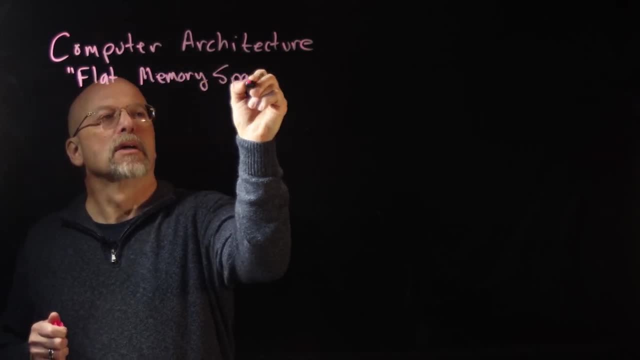 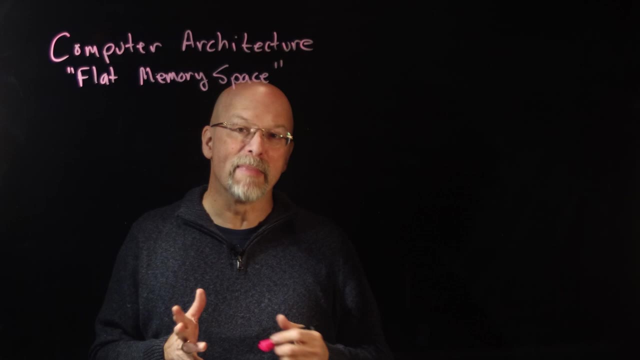 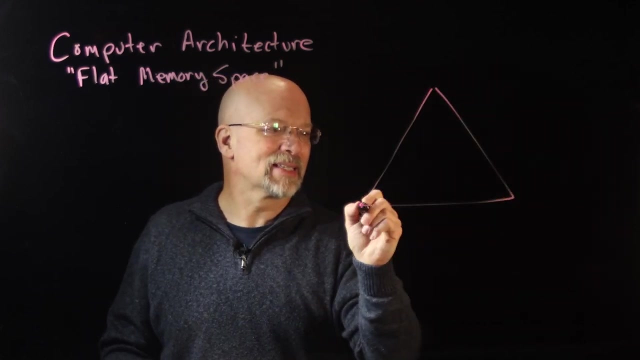 memory space, now flat memory space, is the very simplest way for a computer, for a processor, to interact with a computer with memory, and in fact, let's take a little break and show you a basic. well, it's this, this thing called the memory hierarchy, and the memory hierarchy is: 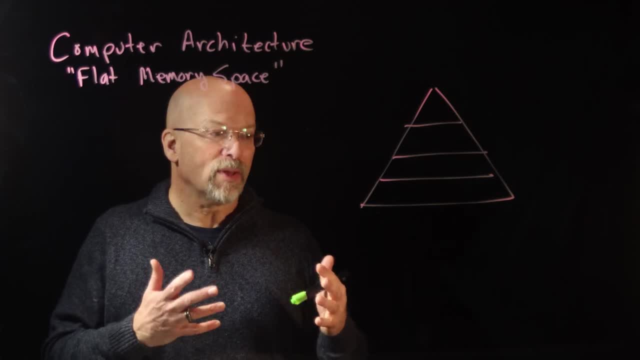 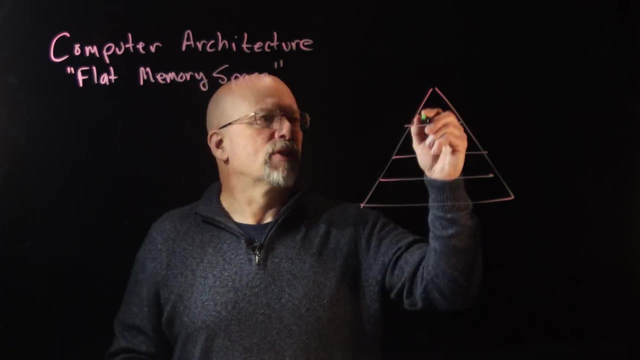 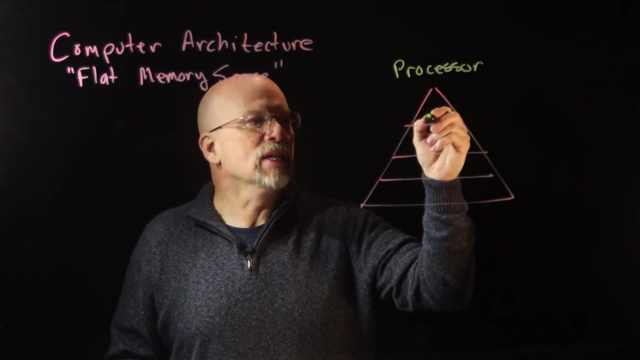 complete, composed of multiple levels where we've got these different components of memory or different places where we can store values. now, at the very top, we've got. well, the processor is sitting up here at the very top. now included in the processor is something called registers. now, registers. 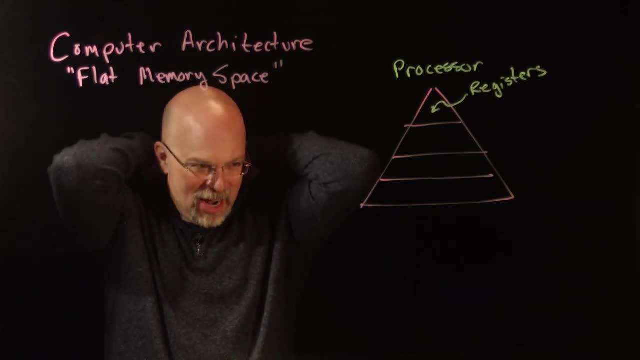 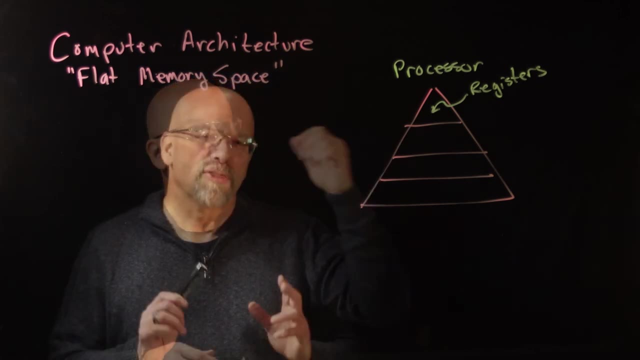 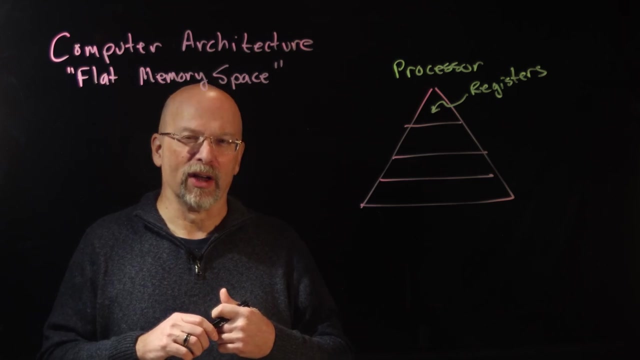 are just groups of those D flip-flops remember, and so you've got the D flip-flops that are storing values and you put a bunch of them together. you can store a larger number. think of it as like a scratch pad memory, so you just need to jot down some notes to remember what you're working on. in fact, maybe a 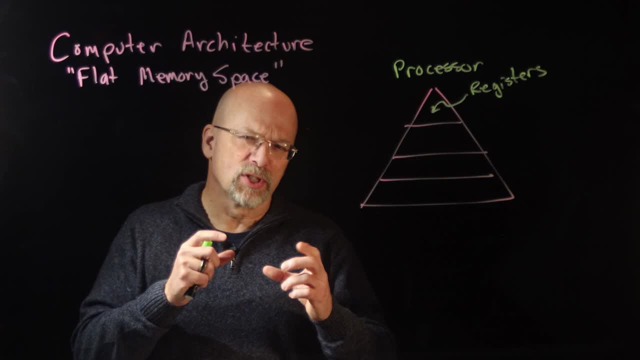 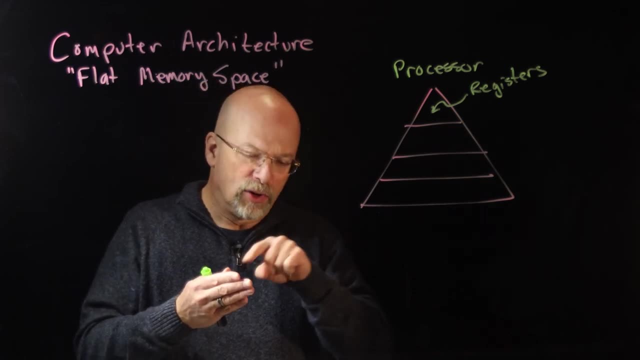 better example of this might be if you've got one of those old-style calculators where you just have a single screen. you know just that one single screen displaying a number, and so you're doing all of your operations, that number that's being displayed on the screen, that's stored in something called. 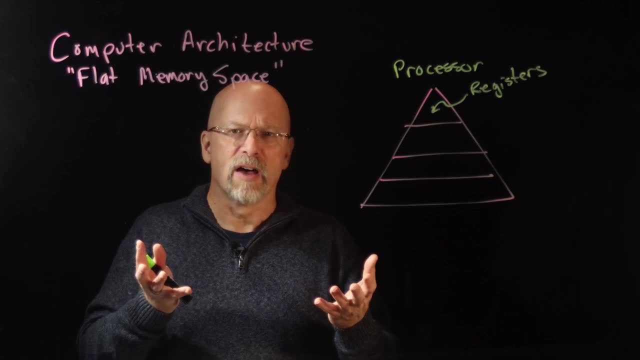 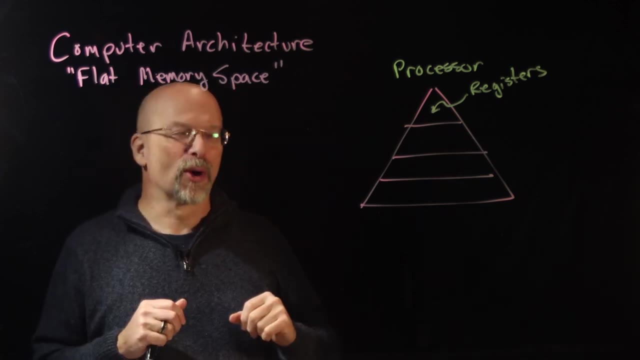 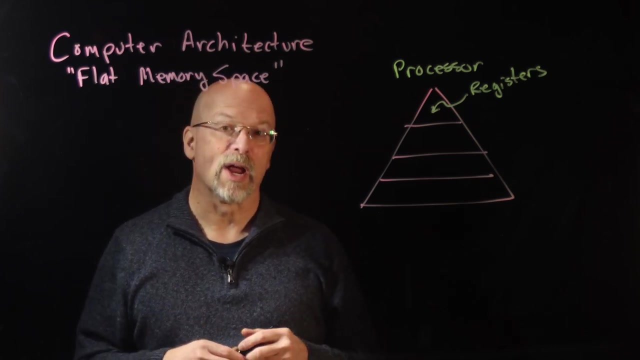 a register. it's basically just displaying the contents of the register. so all the processing, all the computing, all the right now real-time operations that are going on are occurring inside of these registers. unfortunately, we can't store everything that we're working on in registers, so we need to have something that's really fast: a memory. 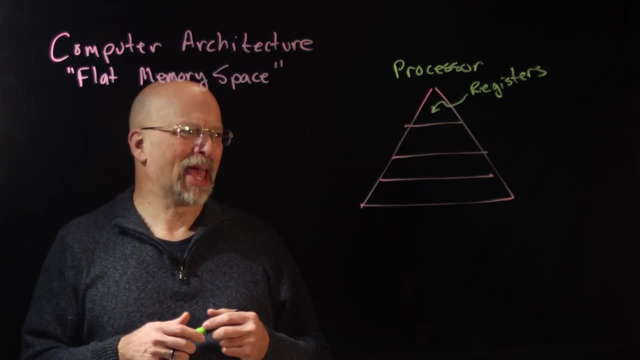 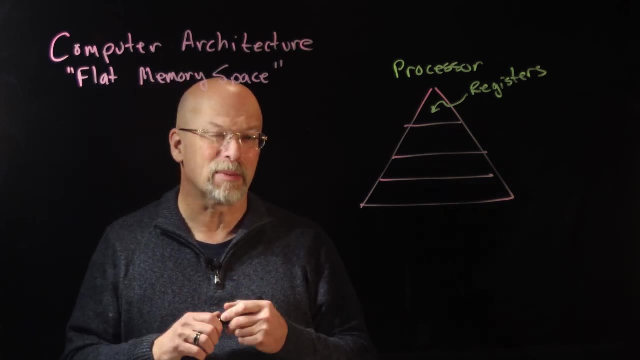 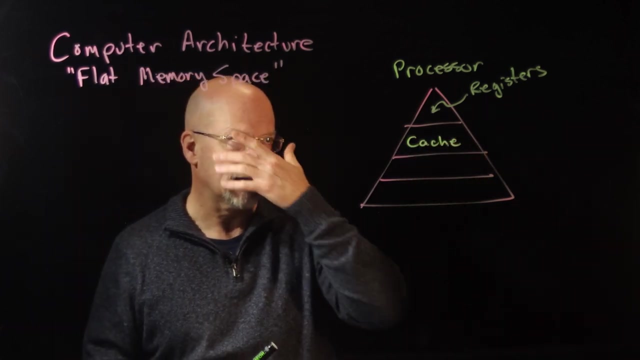 that's really fast but kind of close by, and that's that's still. it's still going to be inside the processor and it's got to be incredibly fast. that's where we have, at this next level, what we call a cache or a RAM cache, and so the 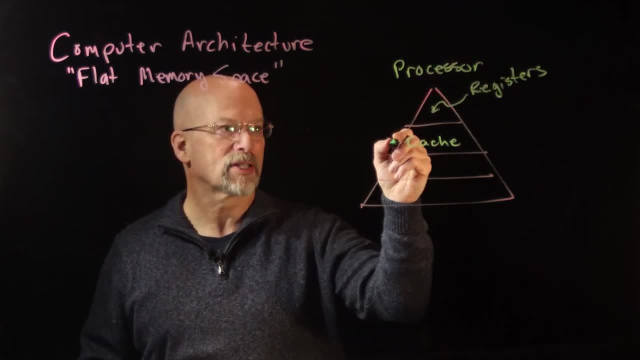 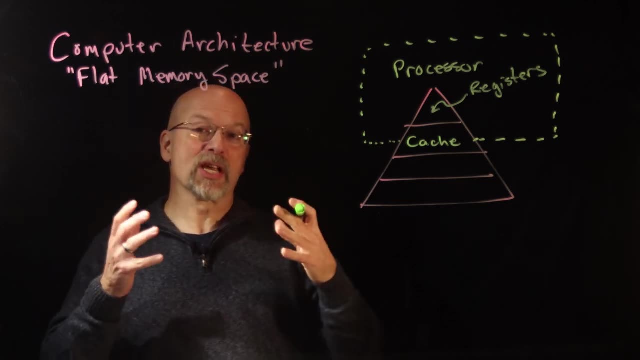 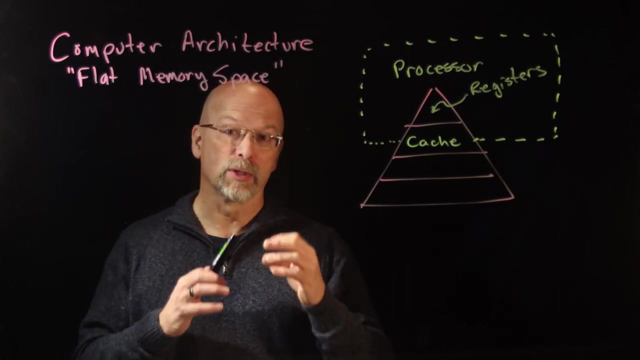 processor and, in fact, a lot of the times, the processor itself can contain some of the cache. there may actually be some cache that is just outside the processor. for example, if I've got a multi-core system, if I've got multiple CPUs on a single, on a single chip, it may be that each one has one of. 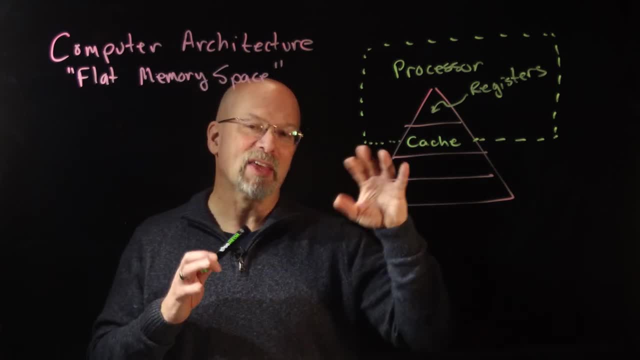 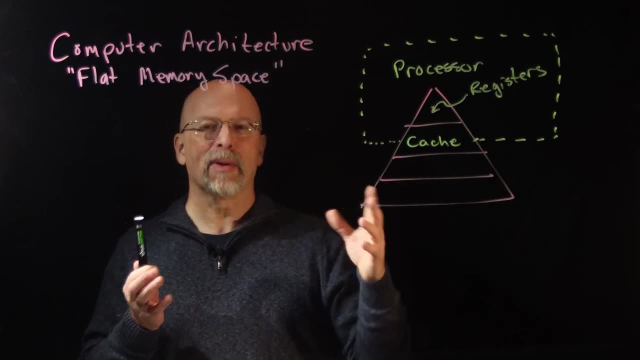 its own, like kind of really close by caches, and then it had. then everybody shares a cache that's a little larger but a little further out that they can share and that might be what's called an L1 and an L2 cache, and L1 cache is the one. 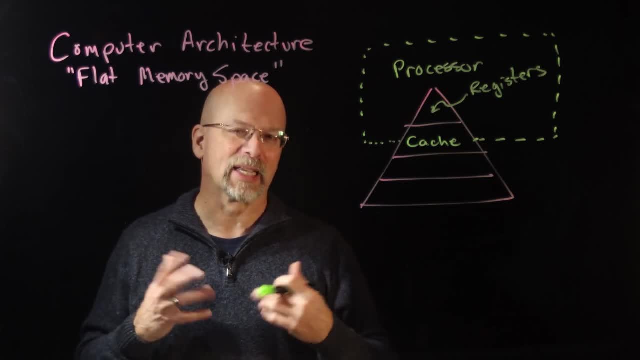 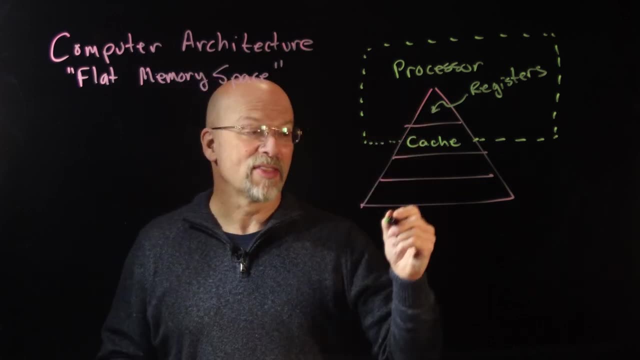 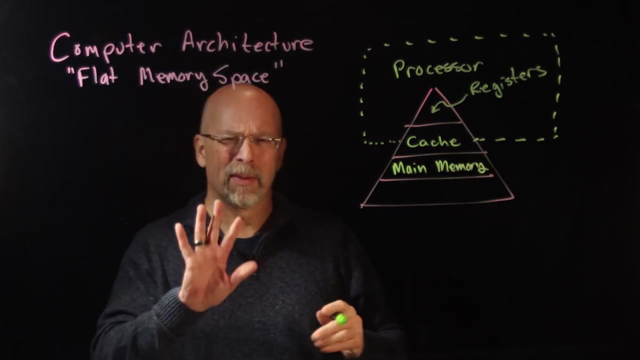 that's inside the processor L2 cache. that's the one that everybody kind of shares. yeah, we have different levels anyway. so you've got these caches now sitting outside the cache, you have main memory. sometimes people call this RAM. RAM is not really the correct term for it, because RAM actually means random. 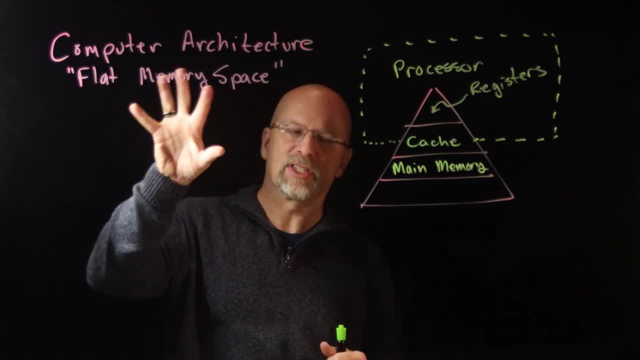 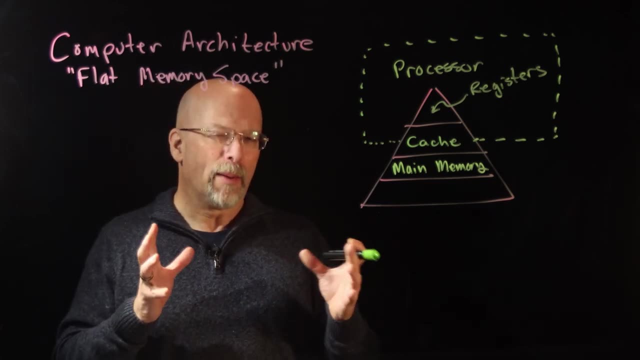 access memory and, in fact, it has a lot to do with this idea of a flat memory space that we're going to talk about in the next lesson, but that's where you're storing, well, pretty much all the active processes we're currently working on. so, for 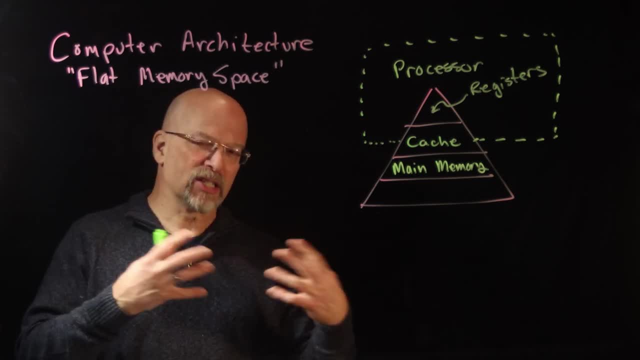 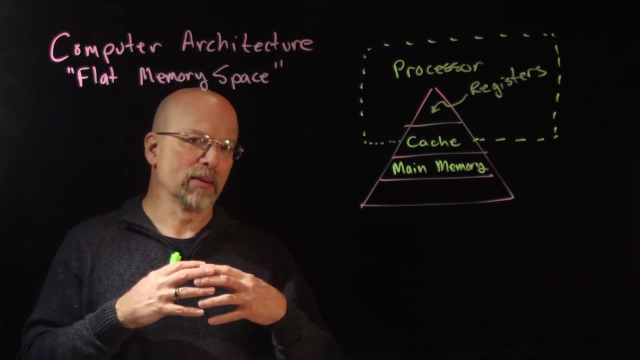 example, if you're running a browser, the certain pieces of software that are active with that browser that you're using with that browser- software that's going to be loaded into main memory. think of it this way: if I have a long piece of code, the piece of code that 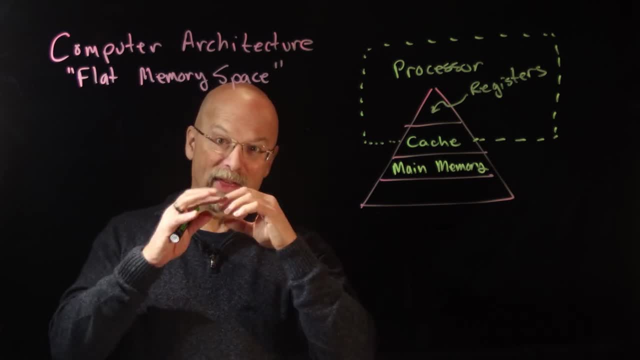 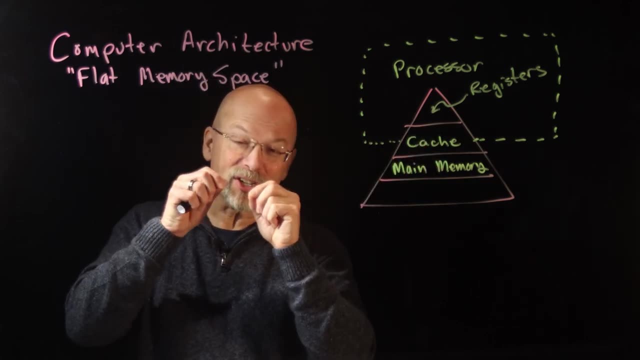 I'm executing is contained in main memory, but the for loop that I'm currently inside of the, the code that I'm currently executing, that may be in the cache, and then the actual instruction, the actual data that I'm working on, those would be in the registers. now we have to have a place to. 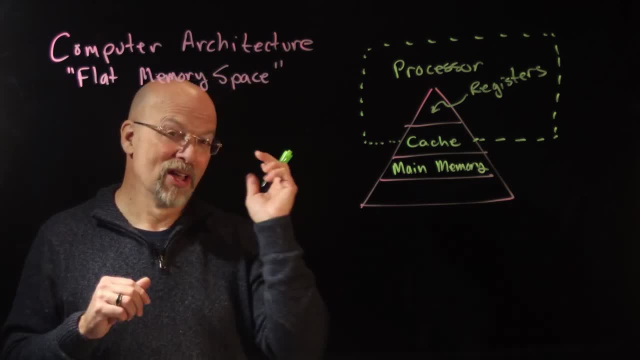 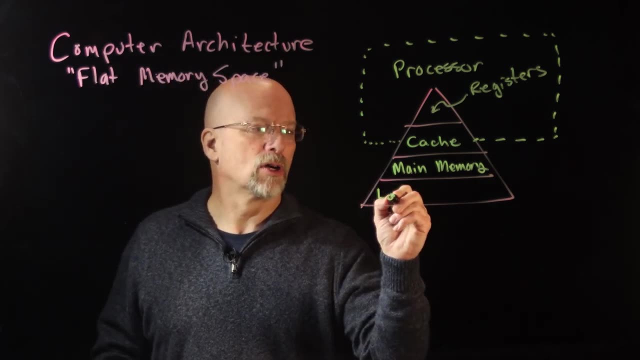 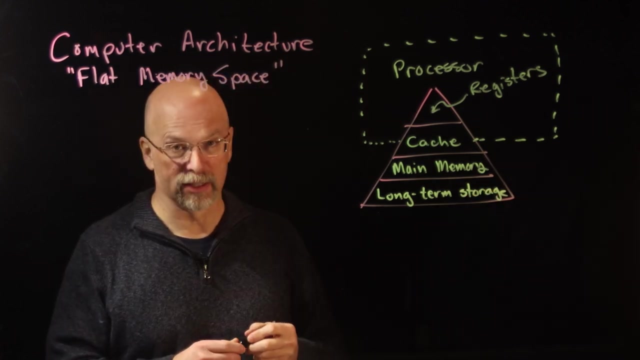 store everything long-term and, in fact, if the machine shuts off, we need to be guaranteed that there is going to be some memory that's kept, you know, accurate, and that's going to be your long-term storage. that is at the bottom of the pyramid and this can include a number of things. it can. 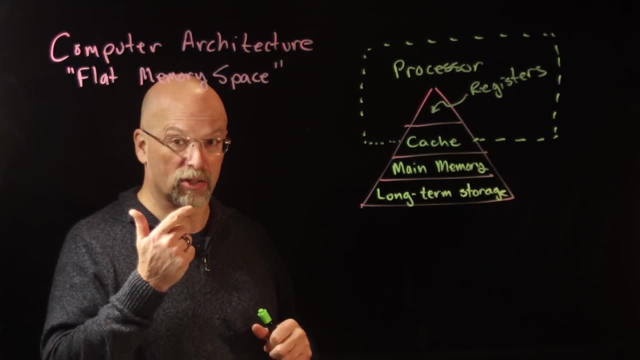 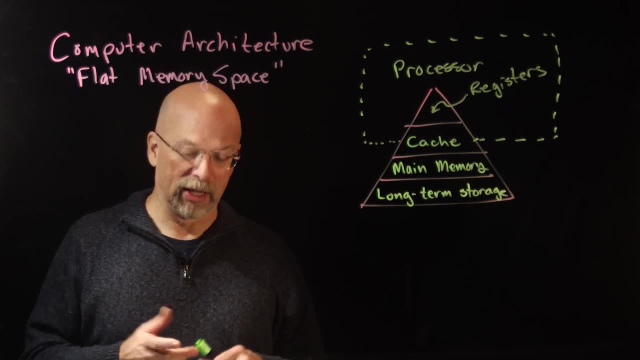 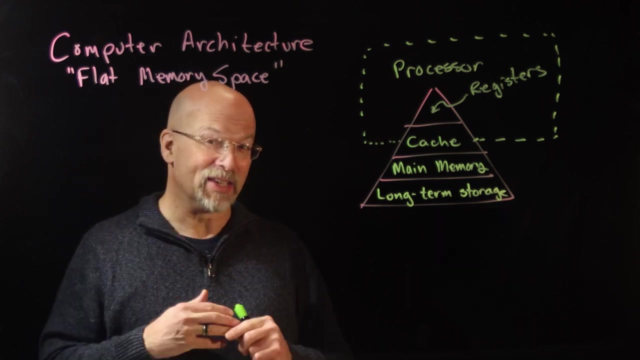 include SSD solid-state drives. it can HHDs, hard, you know, the hard disk or, excuse me, HDD, the hard disk drives. but it can also include things like your optical drives. it can include things like tape drives. yes, tape is still used, believe it or not, because of its long-term store, its capabilities in 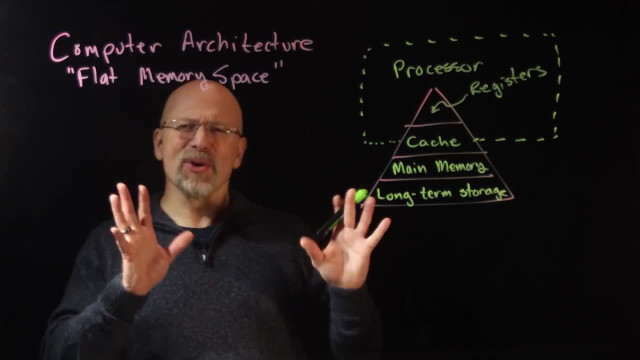 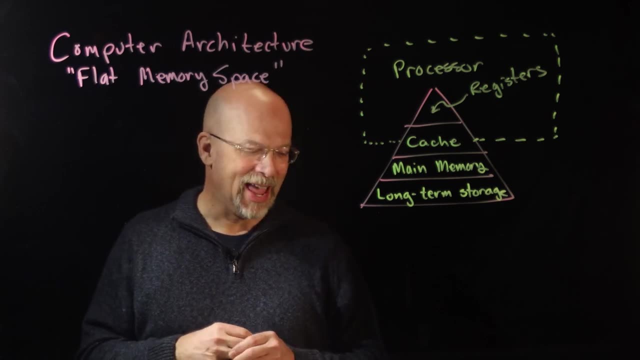 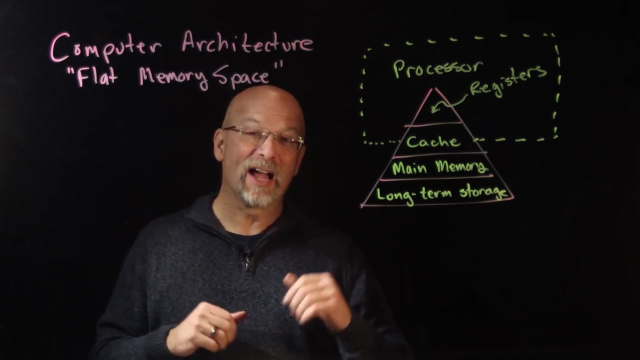 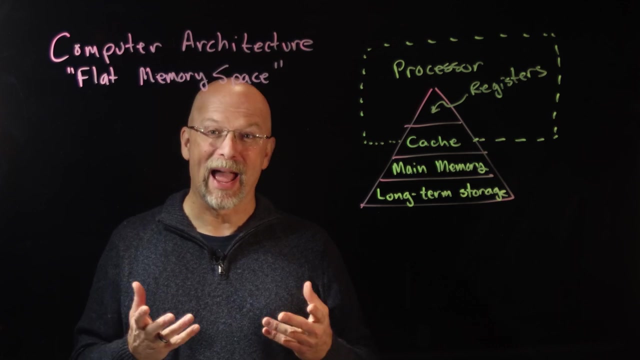 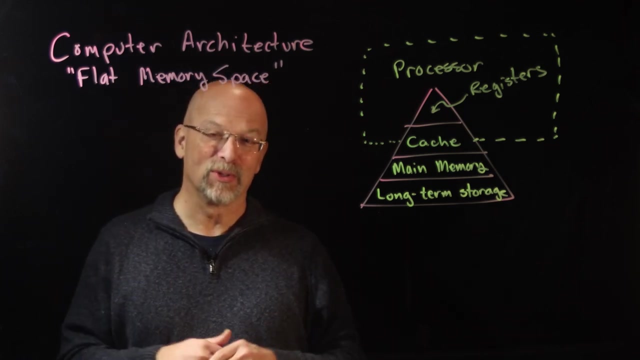 long-term storage. so you know, these define the, the, the, the Trust, Presumable 져. well, not the teenage boy I used to be past, Dave, Let's say that. well, I went through a lot of milk. okay, Now I could, if I had say a bowl of cereal or something I would. where would I first? 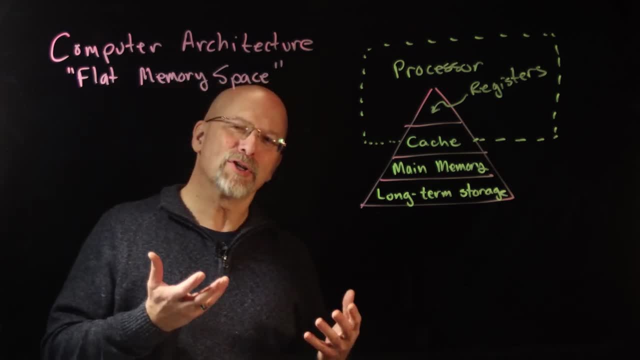 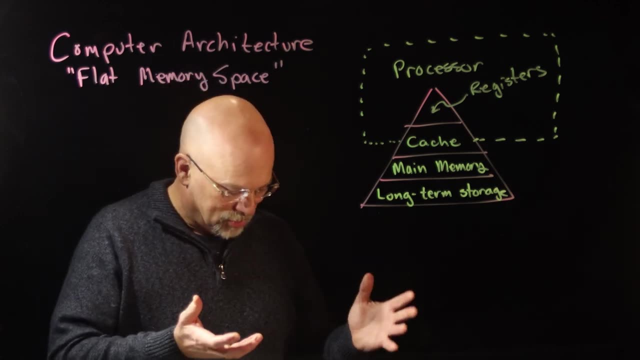 check to see if we had milk. Well, the very first place I'd check to see if we had milk was, well, the refrigerator in the kitchen, right. And so the very first thing you do is you, just you know. 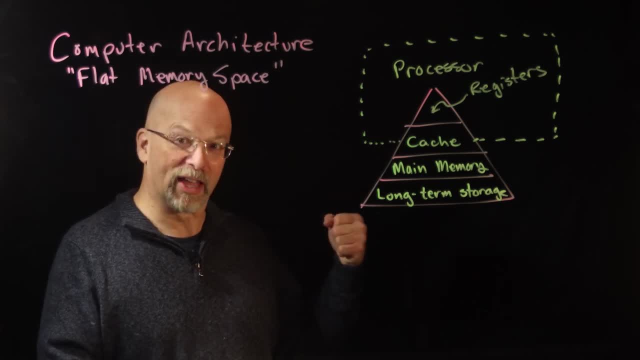 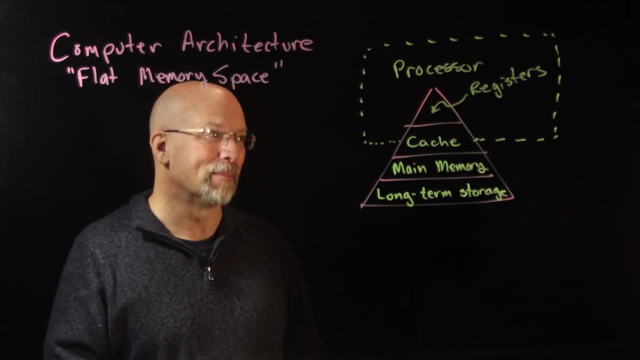 you pour your bowl of cereal, you go to the refrigerator, you open the refrigerator, you take a look. There is what I need in that refrigerator. Am I looking in the registers, so to speak, for my milk? If it's not there, where do I go? Well, we had a couple of refrigerators in the basement. 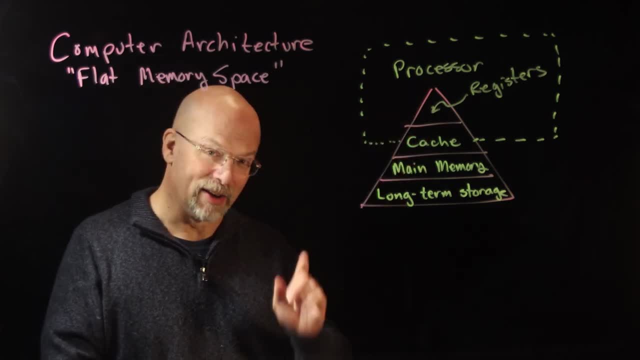 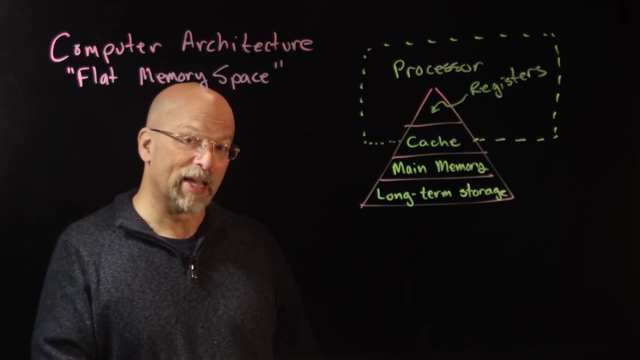 too, And so if I didn't find any milk in there- and mom knew of course she was raising a teenage boy, so she would have plenty of gallons of milk in the house, So I would go downstairs and check in the basement to see if the basement refrigerators had it, I would go to the 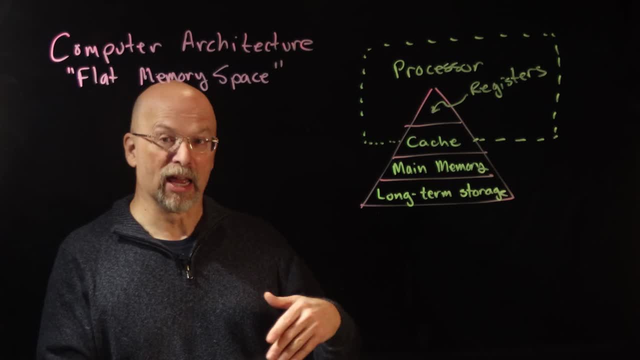 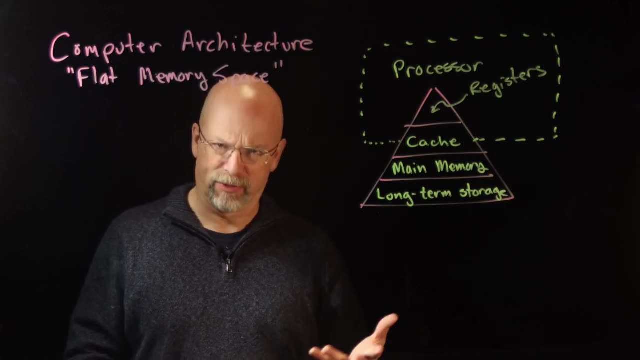 cab And see if the cash was was containing it. Why didn't I go to the cash first? Well, the reason I didn't go to the cash first was because, well, it was farther away, It would have taken longer. I'm 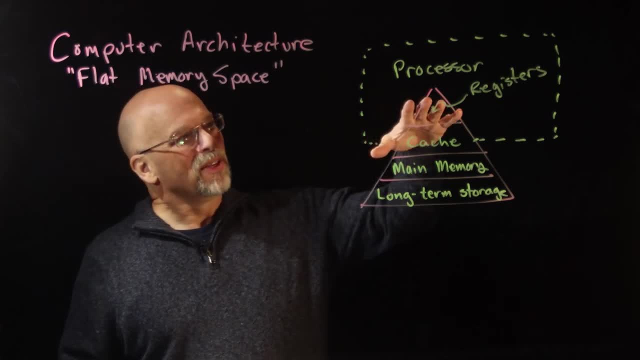 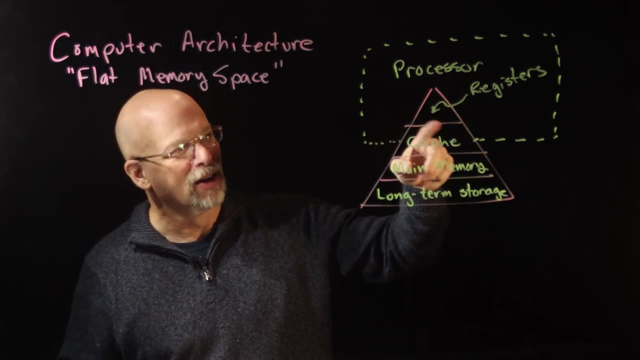 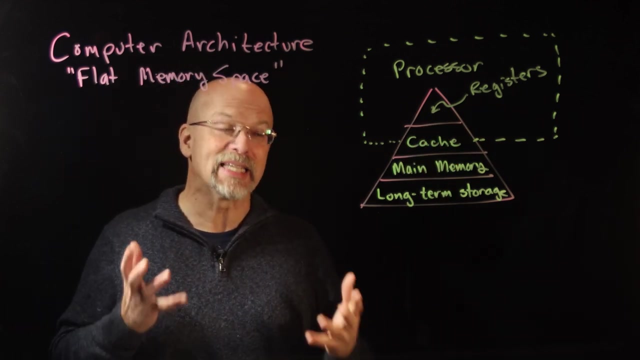 hungry right, And so the fact is is that the cash is further away. But since the cash- and go with me here- I had a couple of refrigerators in the basement. Since the cash is larger, there was a greater chance that it was going to be contained in the cash, And so I would go to the cash and 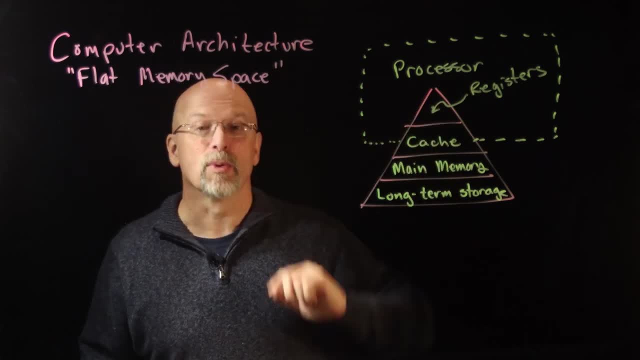 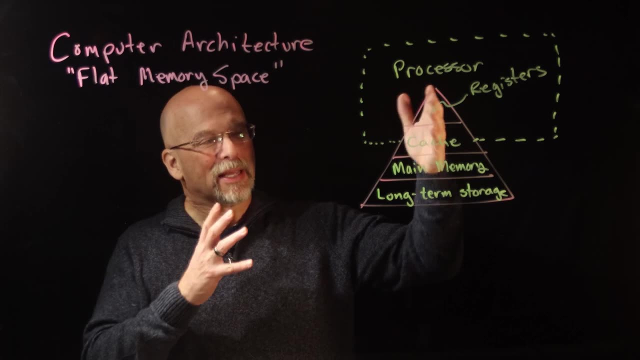 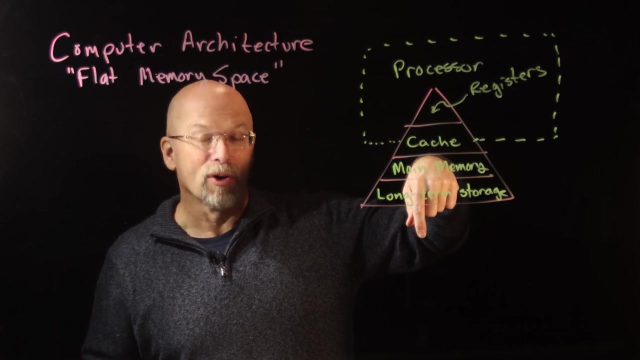 see if the milk was going to be contained in the cash, Then it was possible for it to be contained in the smaller upstairs refrigerator. okay, Also, we were kind of actively. I mean, let's put it this way: So the farther away from where my cereal is, the slower, the longer it takes to find the milk. 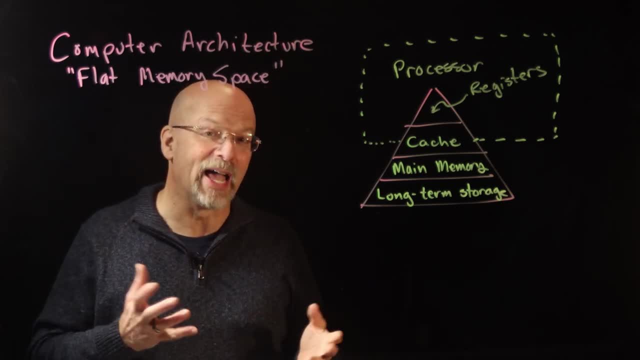 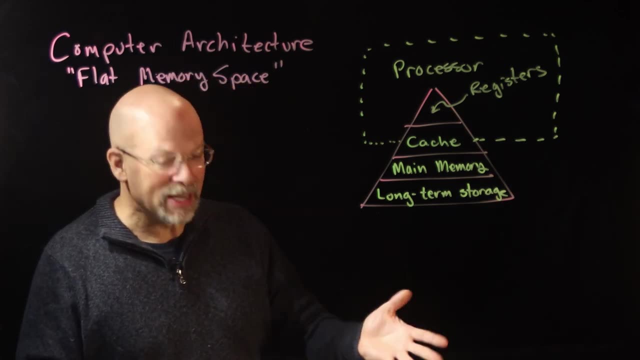 But the farther away I get, the more chance I'm going to find the milk. So next place I'm going to look. Well, let's say that I really want this cereal, But the basement refrigerator didn't have any milk either, Or it went bad, I don't know. 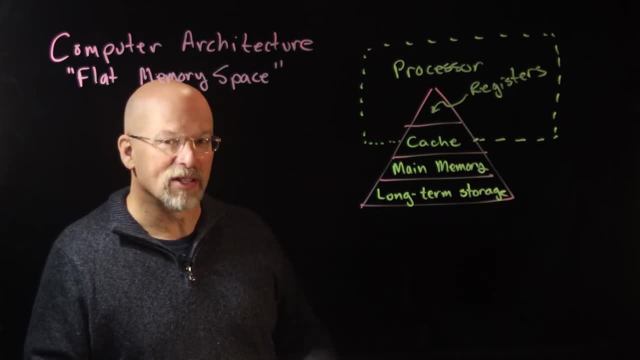 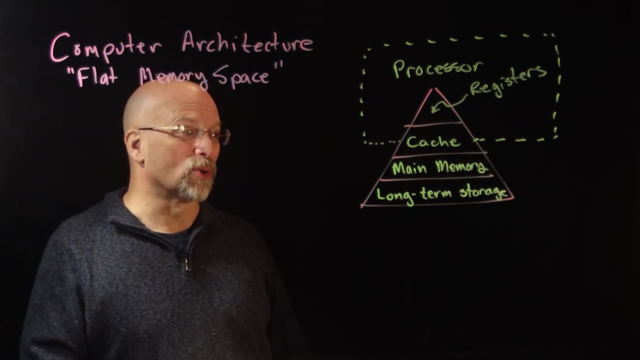 Where would I go next? Well, if I'm really desperate, I would go to the convenience store at the corner right. I would get on my bike or whatever, or drive or whatever, and go to the convenience store. Now the convenience store much larger, much larger, So there's a lot greater. 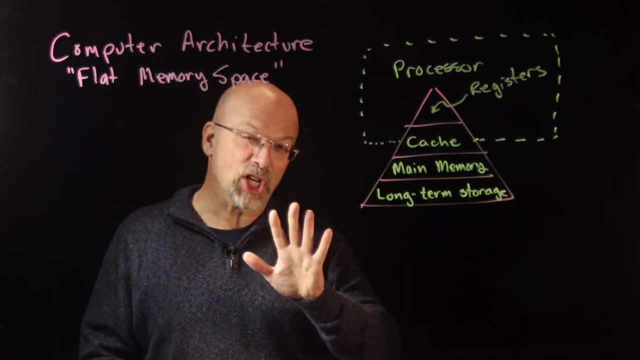 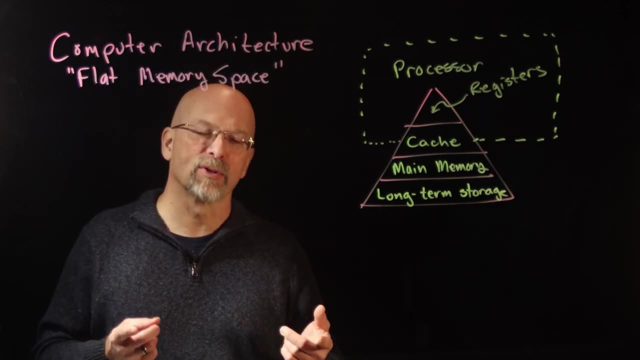 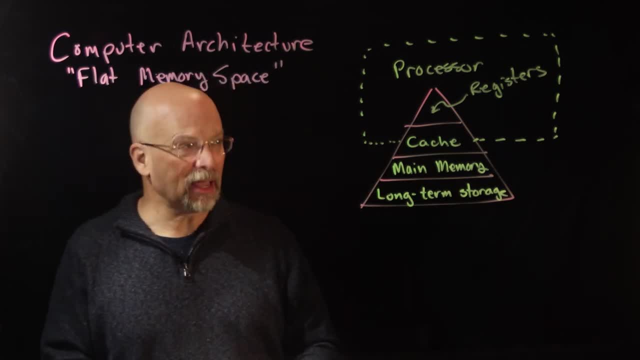 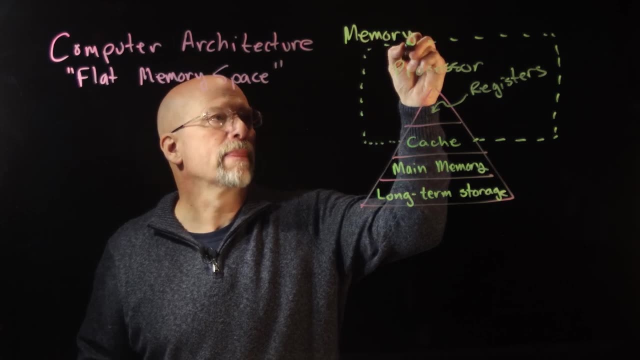 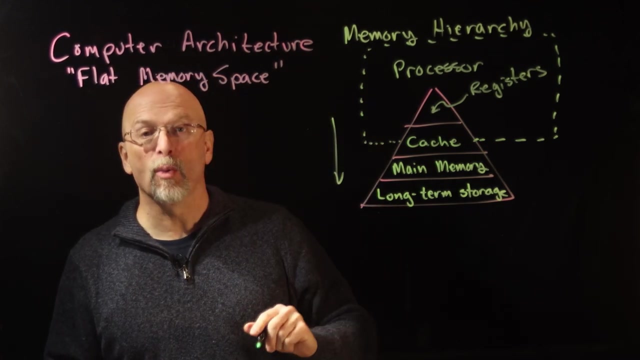 more than likely. yes, it's going to be there. So, if you think about this hierarchy, this memory hierarchy, which is what this is called, this is the memory hierarchy. Okay, Now the memory hierarchy: as you get further away from the processor, it is slower, takes more time, right? So, for example, 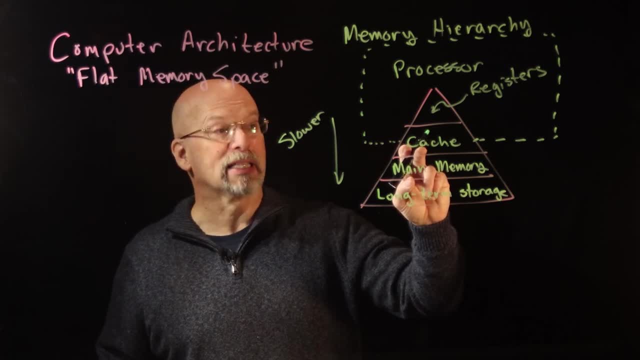 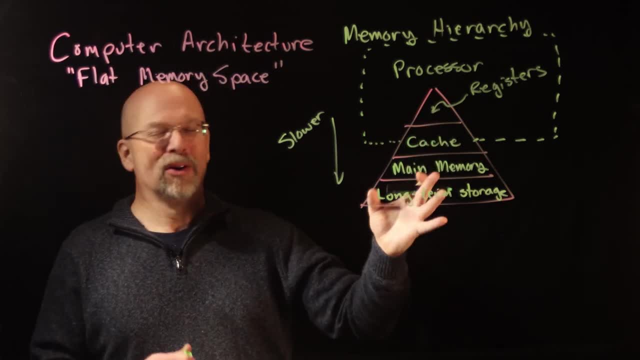 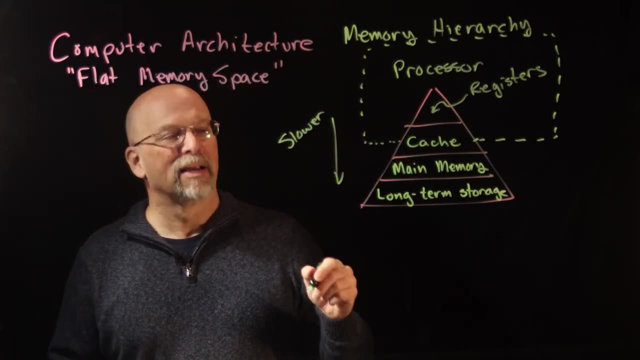 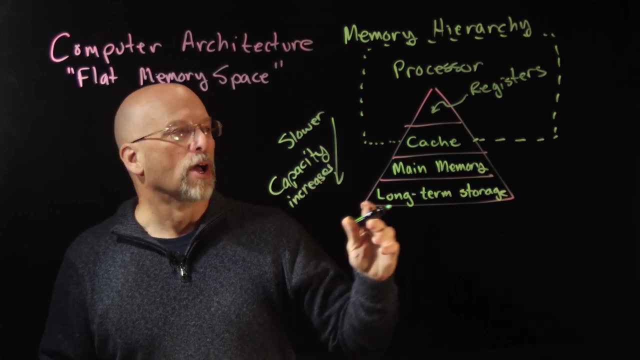 main memory And then you're talking about maybe three seconds or something like that in order to get to the long-term memory. So it's slower to get what you're looking for, But the capacity also increases. So as we get closer to the processor, speed improves. 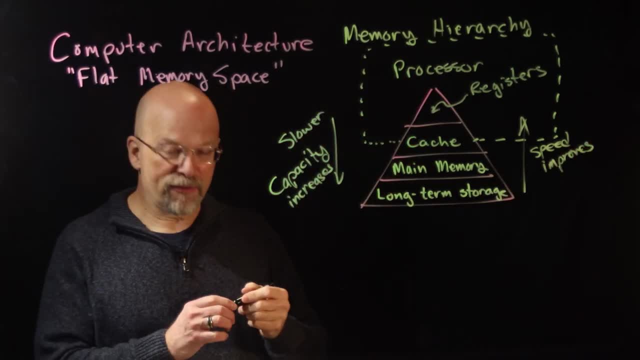 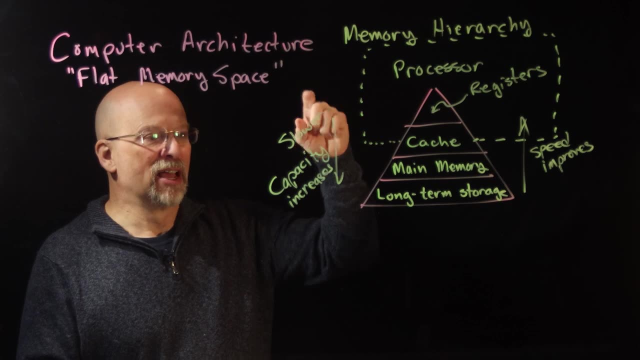 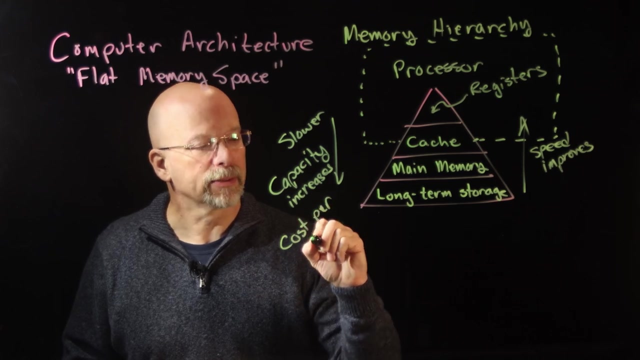 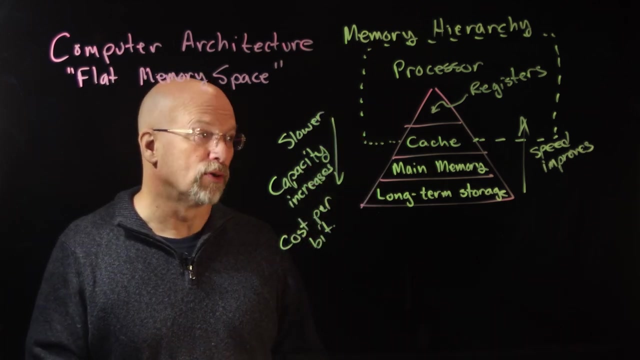 But the chances of finding what we're looking for go down. Now there's actually a third component, a third thing, third characteristic that improves as you get farther away from the processor, And that is the cost per bit for storing data goes down. The cost per bit improves. 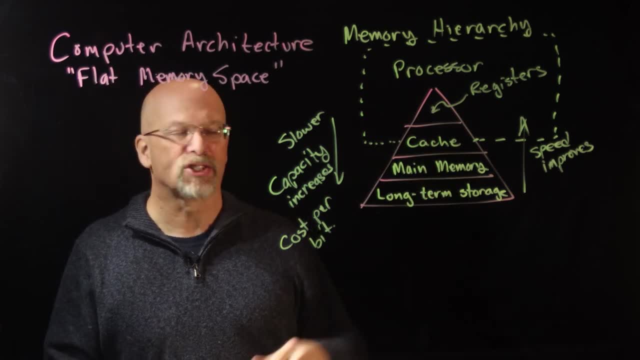 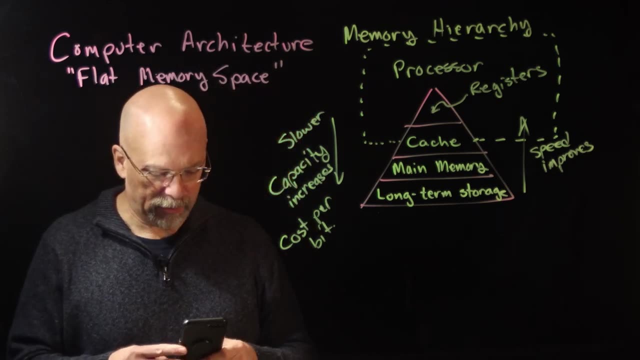 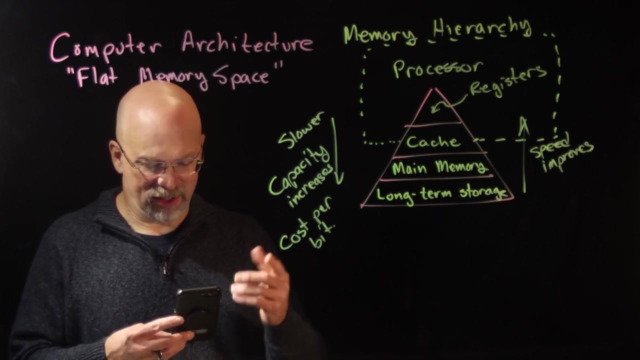 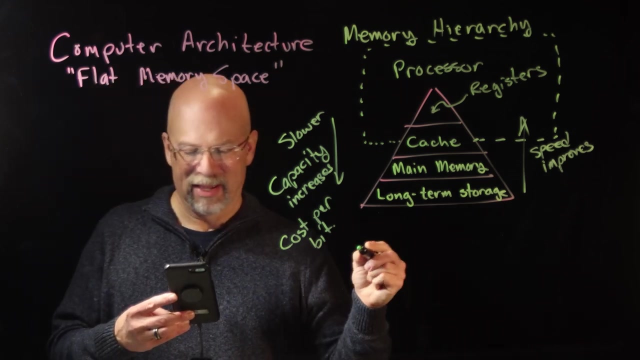 as we get further away. In fact, let's just look at the last two. Let's look at main memory and long-term storage. We could do a really quick search here. So let's look at some memory here. I'm just grabbing something off of the web. How about this? We've got a DRAM. 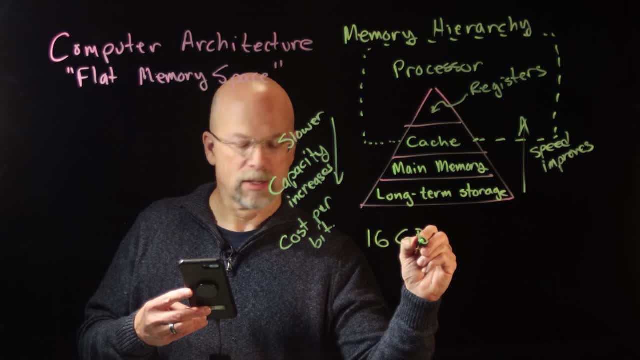 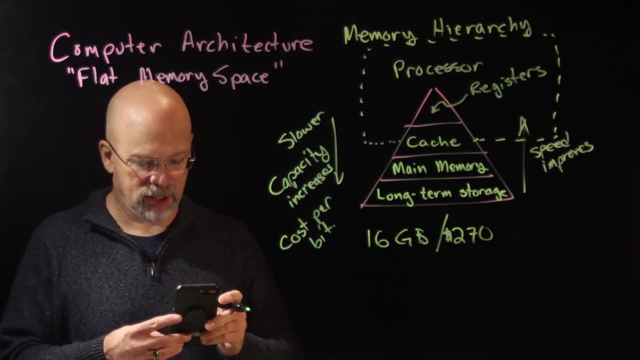 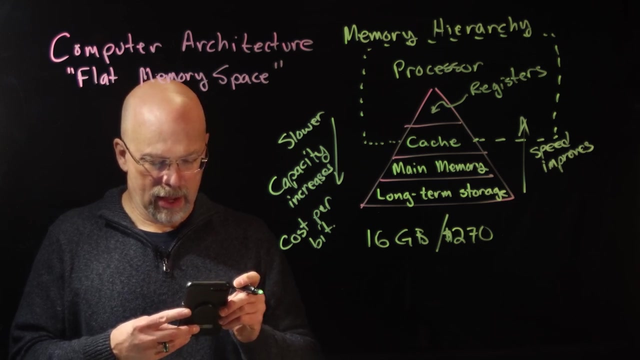 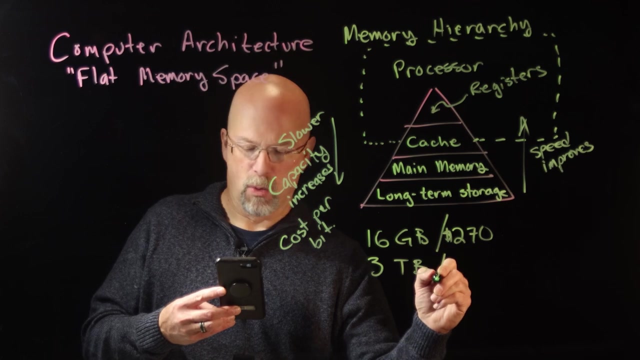 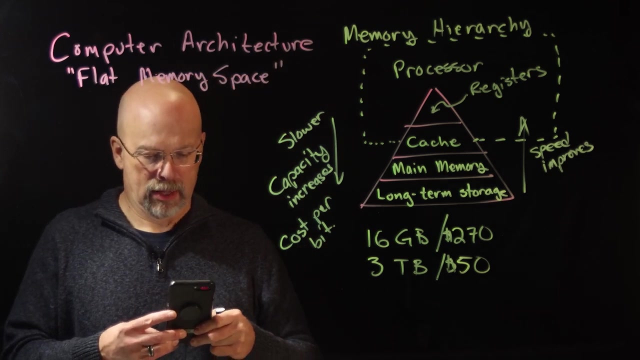 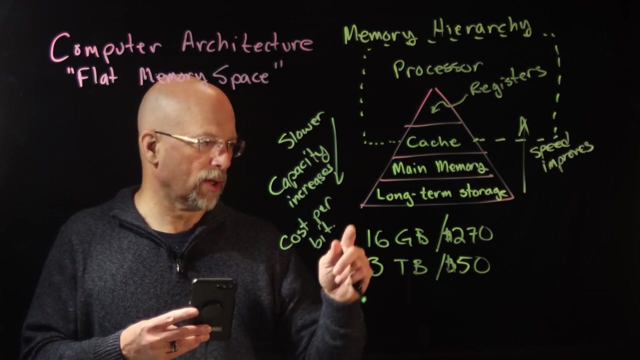 We've got 16 gigabytes for about $270.. Now let's look at the same thing for a hard disk drive. And here we go, We've got a three terabyte for $50,- about $50.. Okay, Now let's take a look and see what the cost per bit is. So if I've got 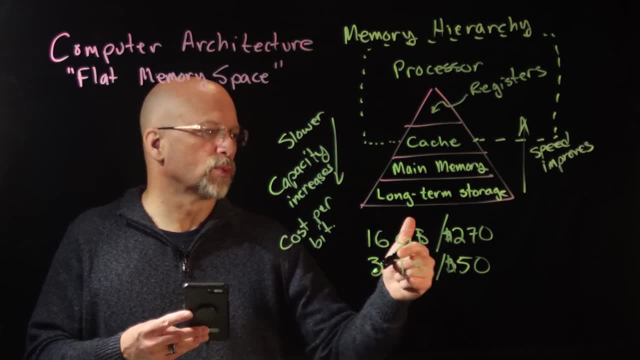 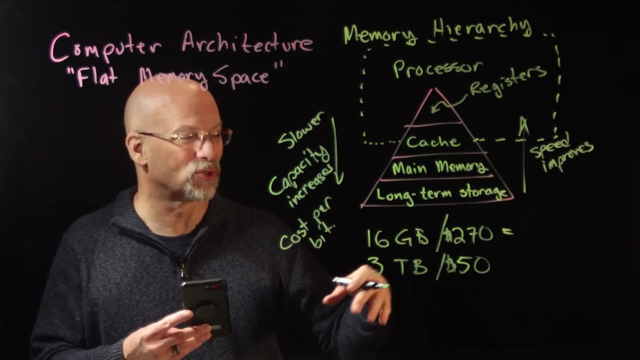 16 gigabytes, And what we'll do is we'll do a cost per, we'll do. we'll do the cost. you know well, in fact I've got my, my, my fractions wrong here, So we're actually going to need. 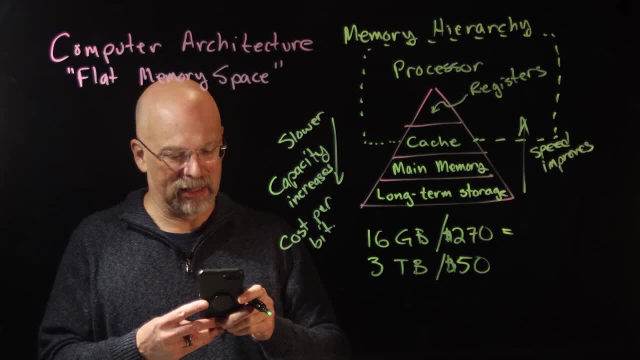 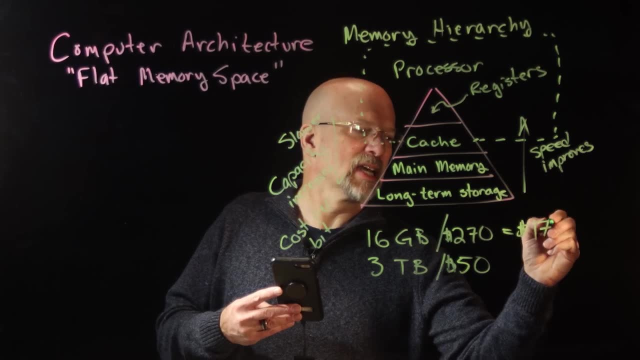 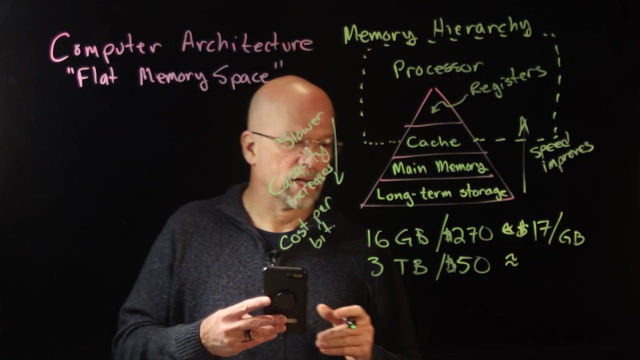 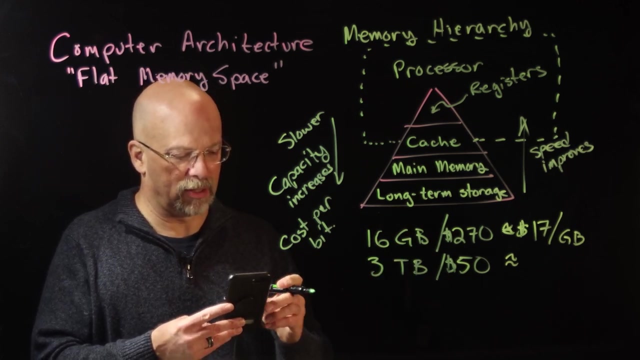 to invert this. So this would be 270 divided by 16 gigabytes. So what you're looking at is about about $17.. So we'll make this about $17 per gigabyte. Now we're going to look at this one. So we've got 3,000 gigabytes for $50.. So $50 divided by 3,000.. 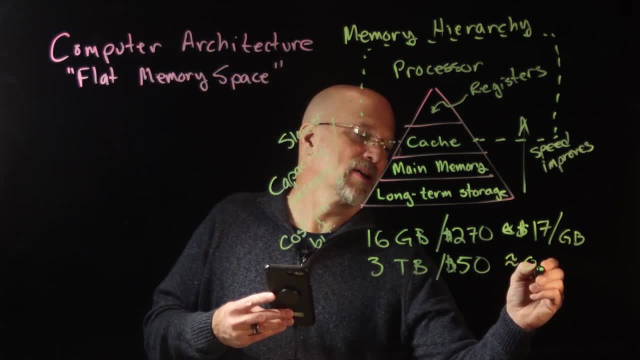 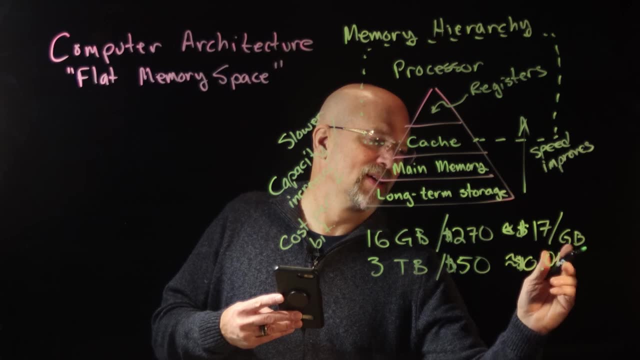 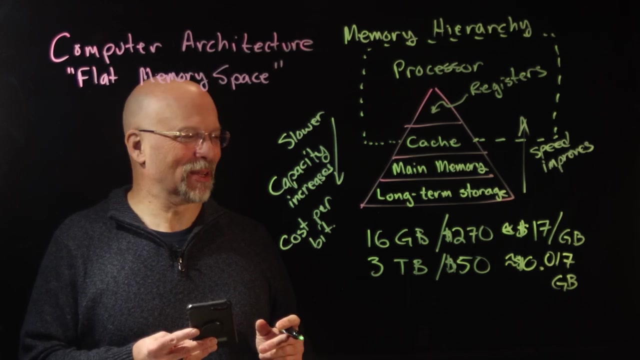 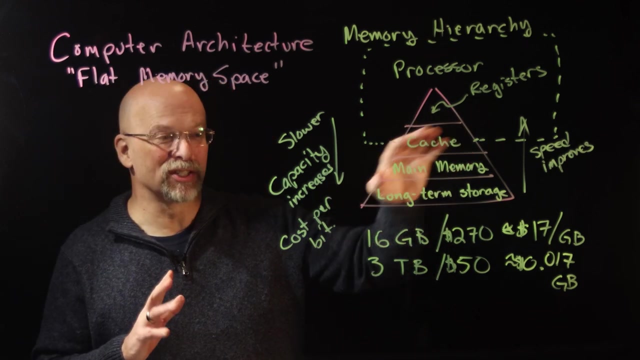 You're looking at about, about what is it I'm doing really well here? You're looking about 1.7 cents per gigabyte, All right, And in fact, people often talk about the technology that's being used to store something. 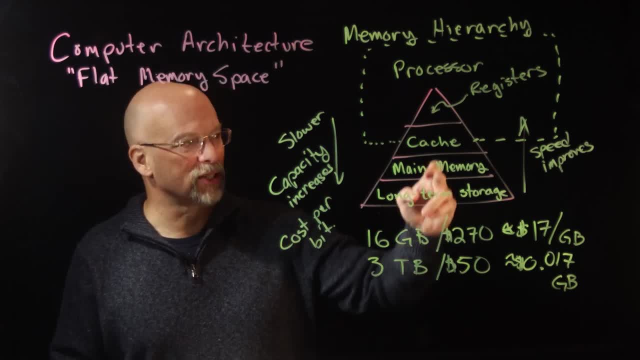 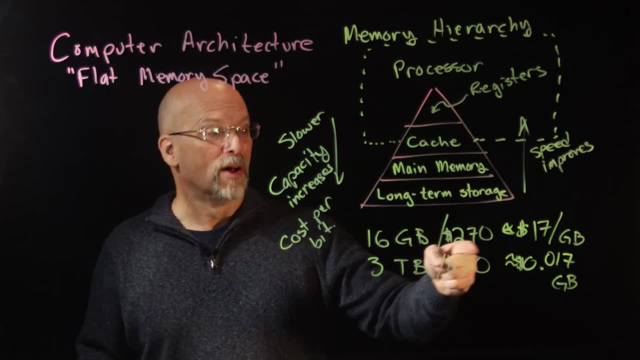 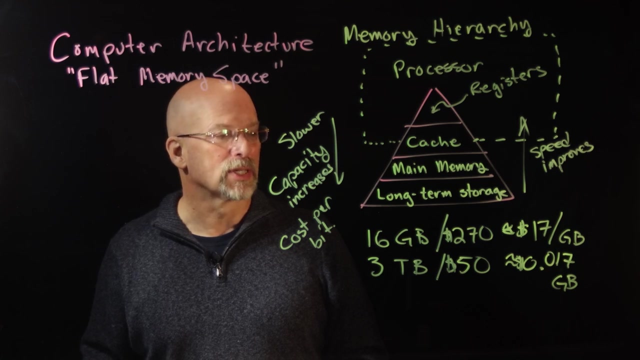 in a RAM cache. Why don't we use the same technology? since the RAM caches are so much faster, Why don't we use the same technology that we make a RAM cache with for main memory? Well, this number right here, the $270 for 16 gigabytes, that'd end up being closer to about $1,000 for 16.